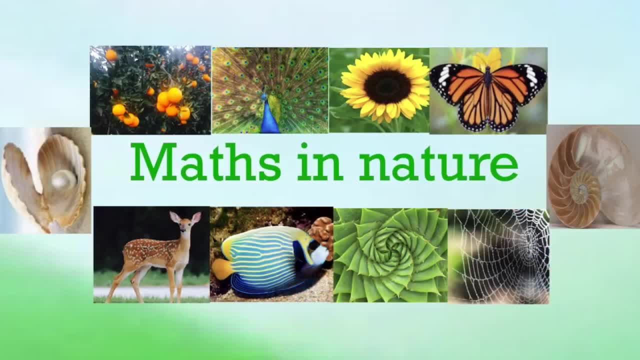 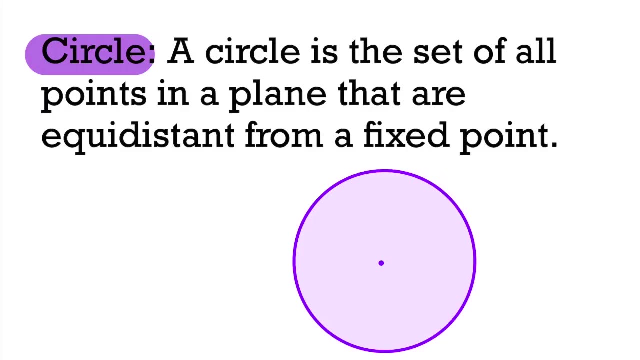 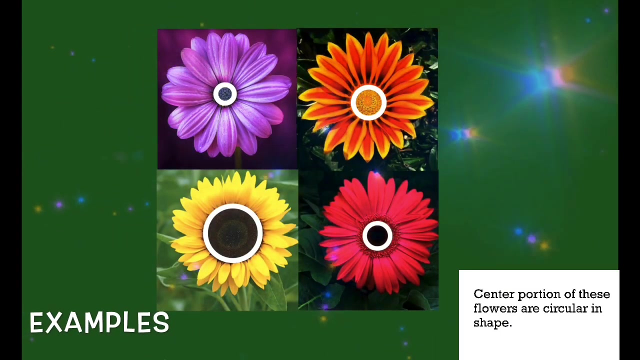 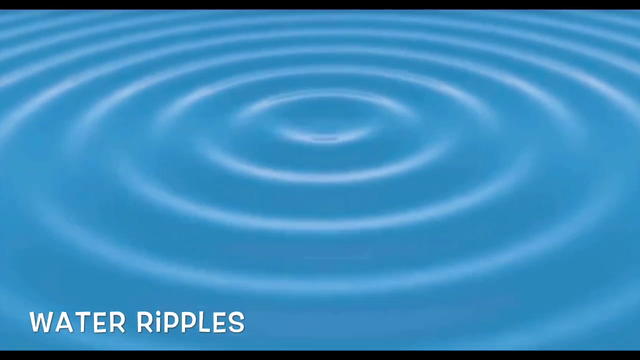 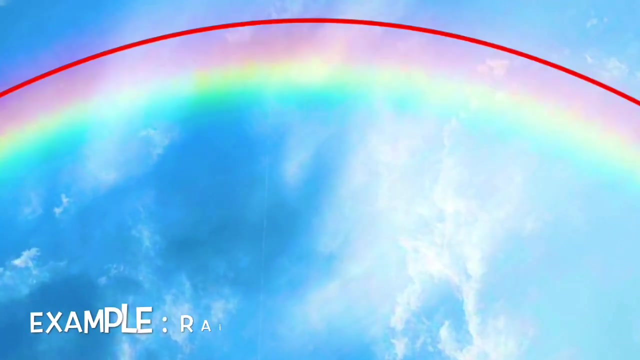 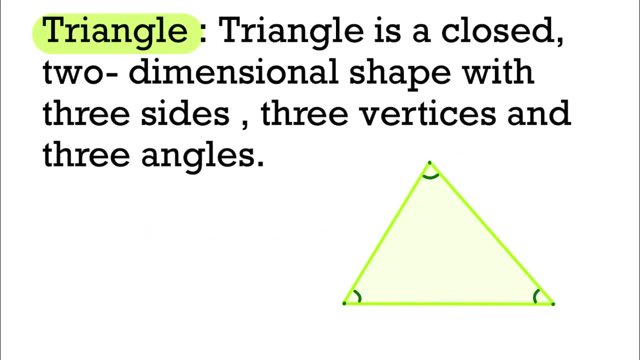 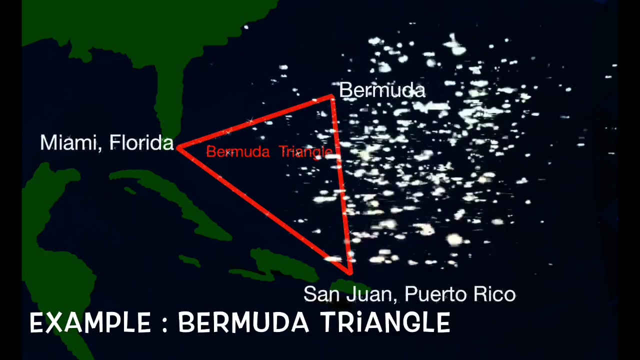 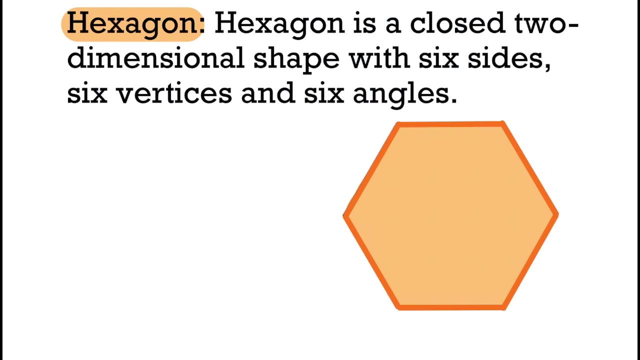 Welcome to Mathworld. Mathematics is everywhere in nature, but we do not often notice it. In this video, I am sharing mathematical shapes and patterns that exist in our beautiful universe. Mathematics is an educational video, but we do not often notice it. In this video, I am sharing mathematical shapes and patterns that exist in our beautiful universe. 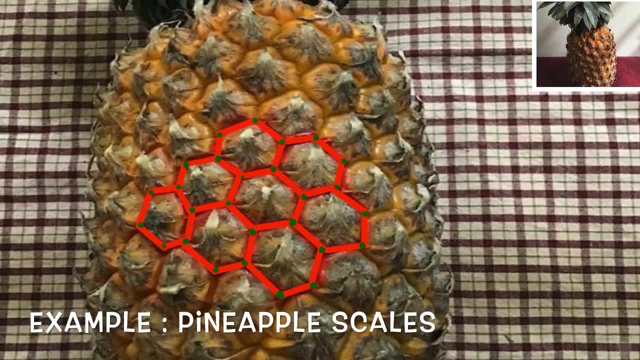 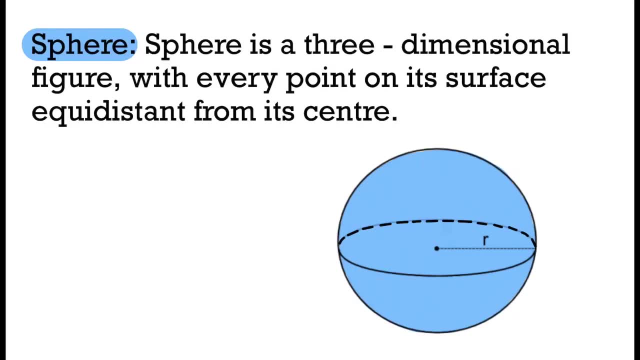 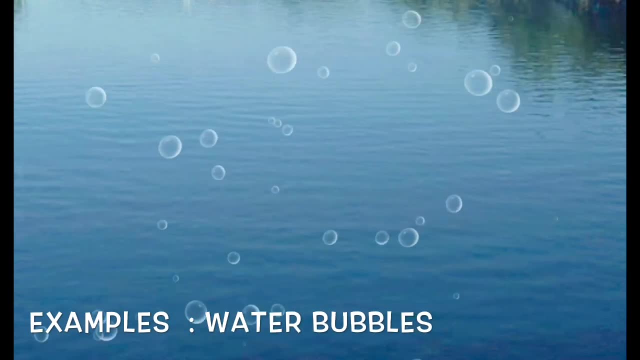 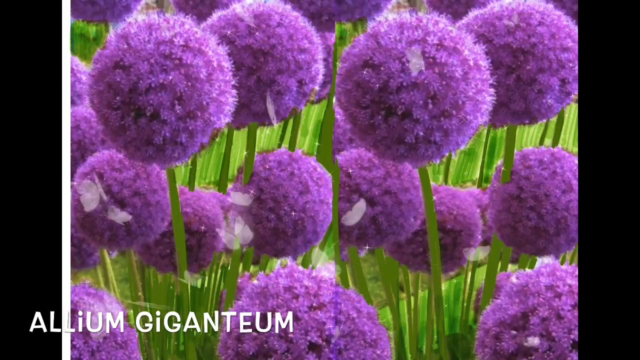 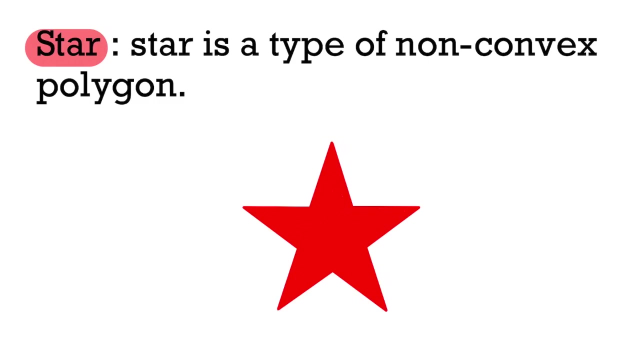 Mathematics is an educational video, but we do not often notice it. In this video, I am sharing mathematical shapes and patterns that exist in our beautiful universe. Mathematics is an educational video, but we do not often notice it. In this video, I am sharing mathematical shapes and patterns that exist in our beautiful universe. 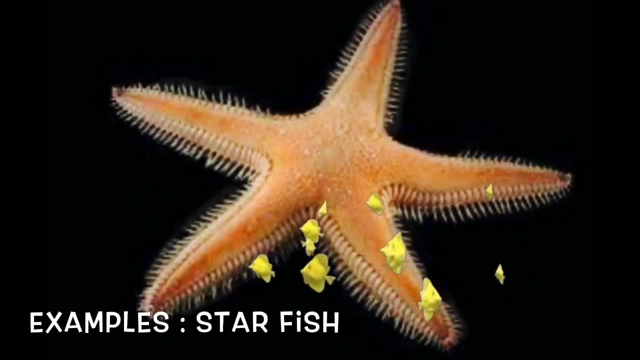 Mathematics is an educational video, but we do not often notice it. In this video, I am sharing mathematical shapes and patterns that exist in our beautiful universe. Mathematics is an educational video, but we do not often notice it. In this video, I am sharing mathematical shapes and patterns that exist in our beautiful universe. 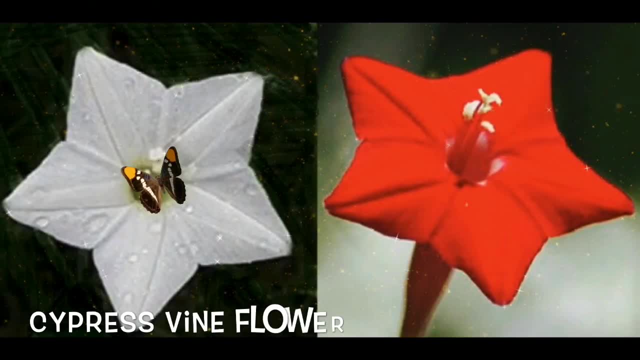 Mathematics is an educational video, but we do not often notice it. In this video, I am sharing mathematical shapes and patterns that exist in our beautiful universe. Mathematics is an educational video, but we do not often notice it. In this video, I am sharing mathematical shapes and patterns that exist in our beautiful universe. 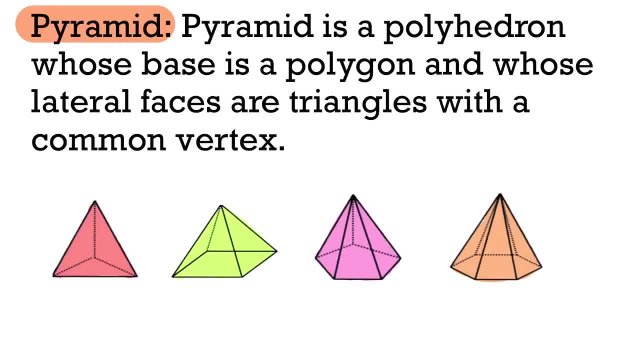 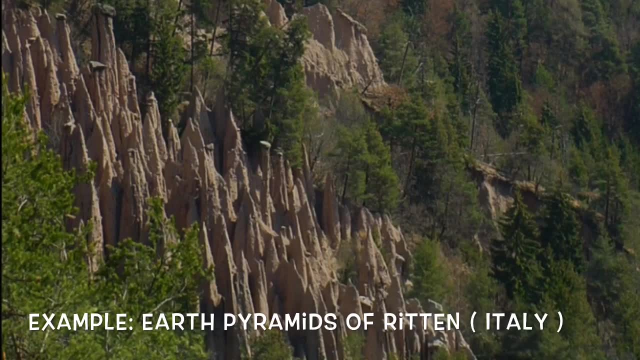 Mathematics is an educational video, but we do not often notice it. In this video, I am sharing mathematical shapes and patterns that exist in our beautiful universe. Red cruising in high five. I get red lost up on hard drive. It's red cruising in high five. I get red lost up on hard drive.